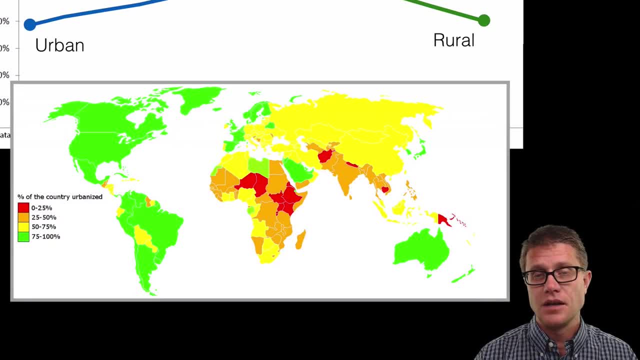 going to flip flop And so we are getting this movement. We are going to see a lot of this movement to the cities. This has already occurred in a lot of the developed countries, And so the US. it is already over 75% of the people are living in the cities, But we 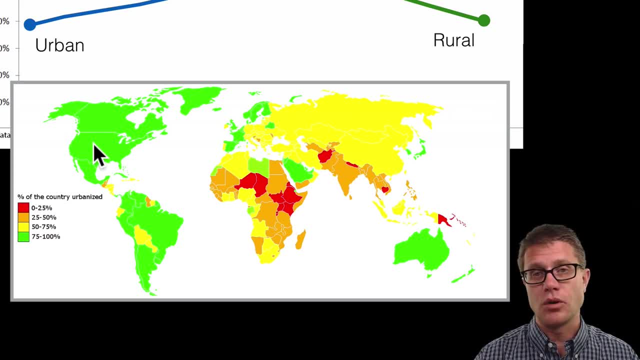 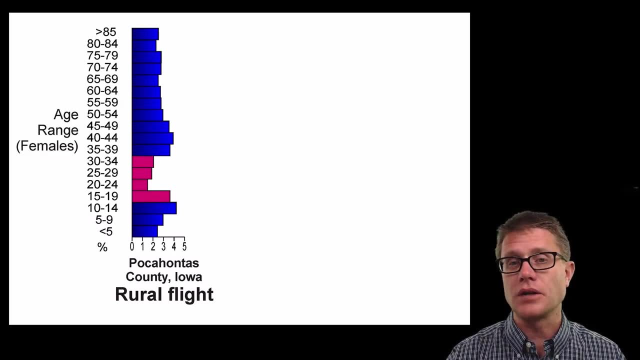 are going to see this in developing countries. As they come online, we are going to have more people moving into the urban areas. You can see this in an age structure diagram. This is females in a rural county in Iowa And you can see that once they go to college, the 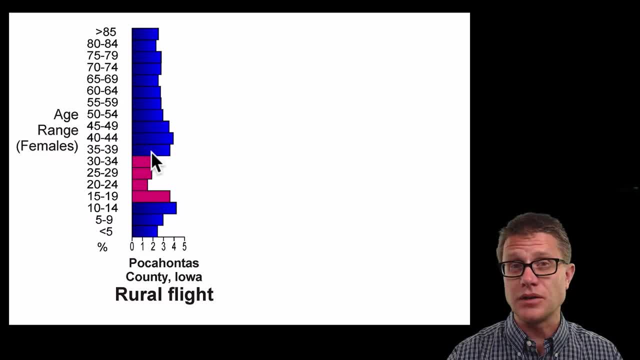 numbers drop off in that area. Now why is that? In a rural setting with industrial agriculture, there are not jobs anymore, And so you can see that they are moving into the cities. This is the growth in an urban area of Iowa, And so we are seeing this movement into the 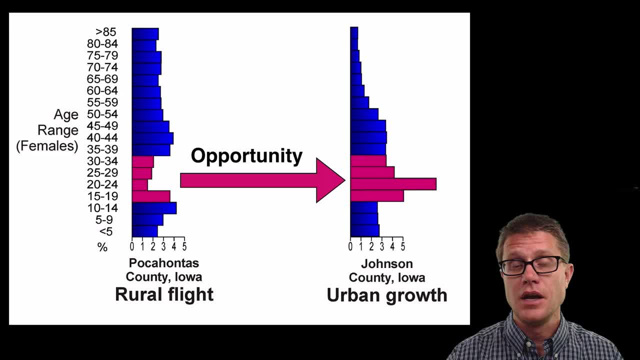 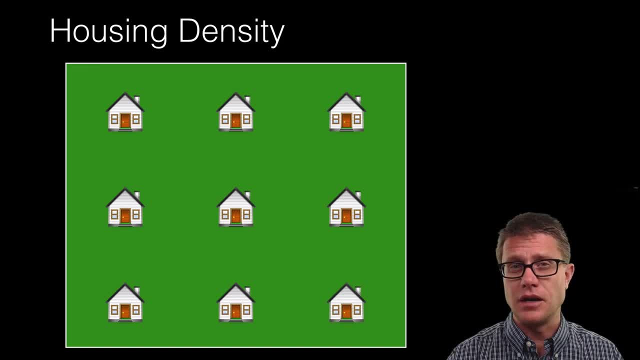 cities due to opportunity. You can get jobs there, And once you move into the city, you are not going to move back, And so this transition is going to occur into the future. It is actually a good thing If we think about low density housing. I want you to concentrate on the 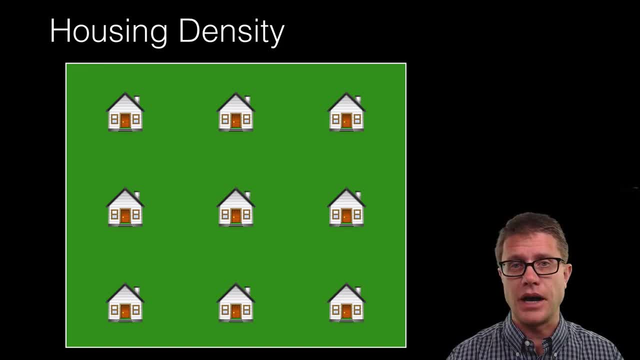 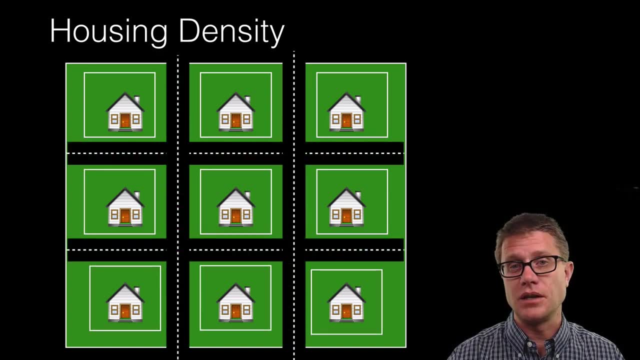 green area here. Let's say we have nine houses and they are all spread out. Let's say this is in a subdivision. Each of them have their own yard. Then we have to put roads to each of those And what is happening is we are losing that valuable land. But if we get the 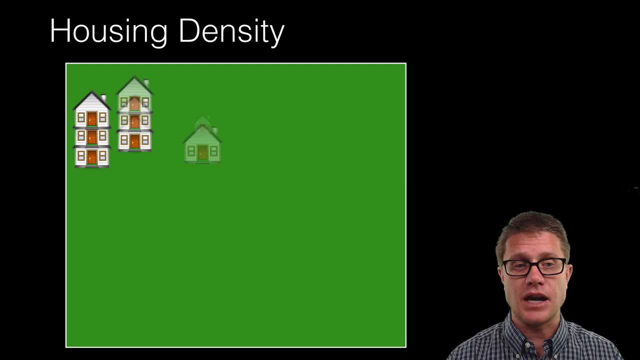 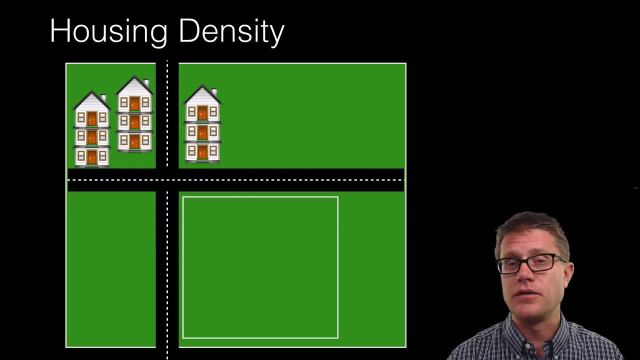 movement into the cities. so we take those same nine houses, stack them on top of each other. let's call them apartments. now we have got higher density housing, We can have a park that they share and fewer roads, And now we leave more of that land outside the 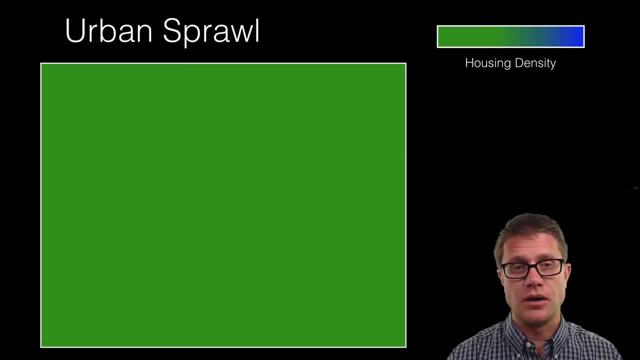 city, And so cities are actually good. The problem is urban sprawl. And so if we put a city right here And then put a couple of roads to it, So back around the turn of the last century cities started to grow And that is because there were opportunities there. And so if we say 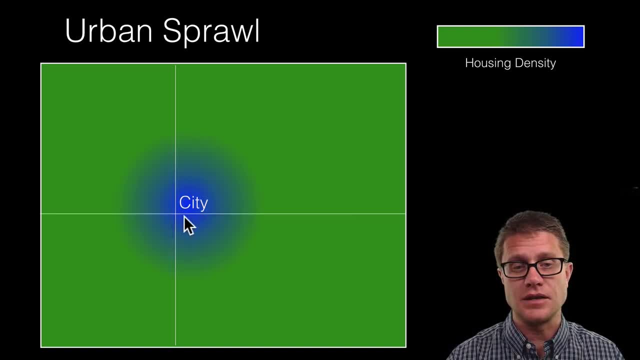 this is the housing density, So we are going to have the greatest density inside the center of the city. There is opportunities there. It is really hard to get into the city. We do not have a lot of roads, We do not have a lot of transportation. It is hard to get. 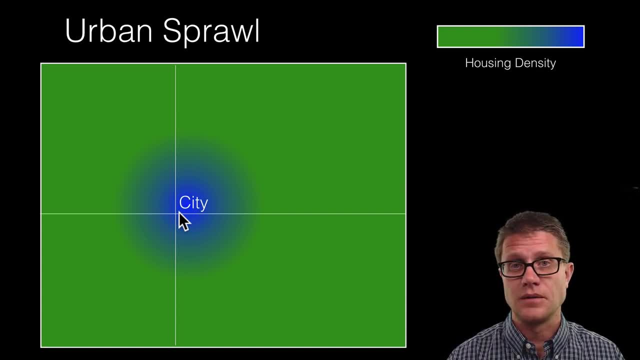 out of the city, And so we are going to see these flourishing inner cities. Now, what happens, though, around the last half of the last century, is that we have the arrival of roads, And we are going to see these flourishing inner cities. Now, what happens, though, around the 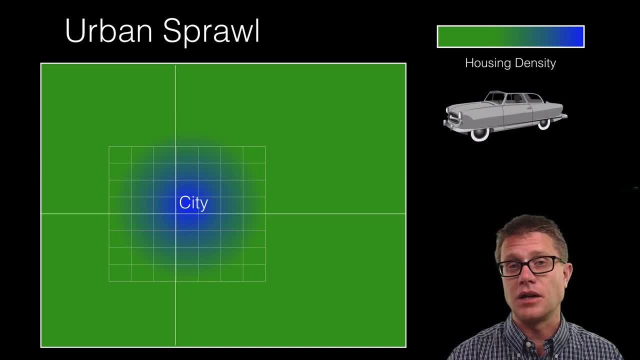 last half of the last century is that we are going to see these flourishing inner cities, And so the result is that the city is getting faster, And that is because of roads, infrastructure and the automobile. Now it is easier to get in and out of the city And people started 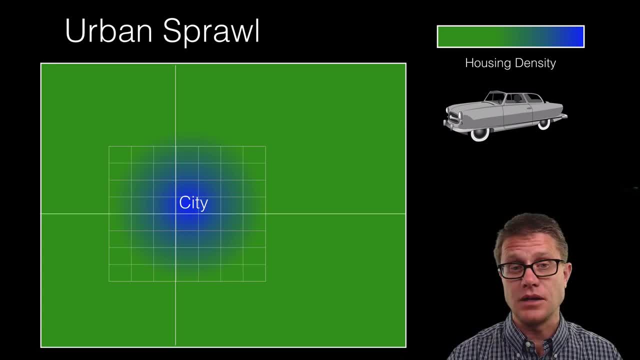 doing that, They started buying up lower density housing, And so what you get is this urban sprawl, This movement away from the city, And this is a positive feedback loop. The more people move out, the more roads there are, the more tax base there is, and we are. 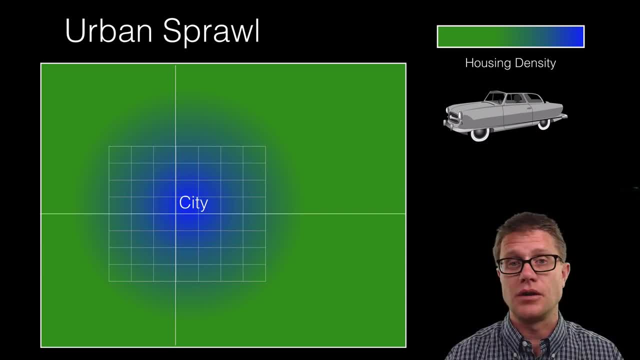 going to get more movement out And we are going to encroach into the area around it. They are also bringing their tax base with them, And so that leaves a lot of the time urban blight inside of the city where people are not actually living. Now this is kind of a United States. 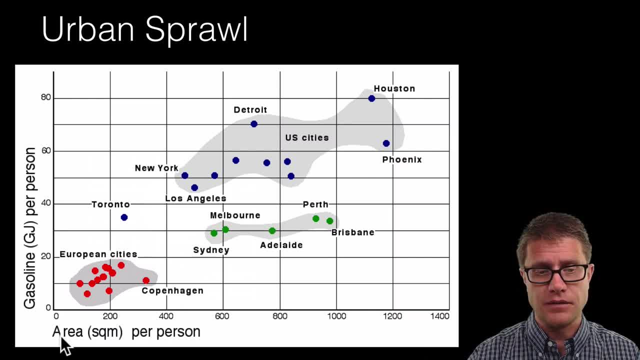 problem where it is more of a problem in the US, And so if we look at this graph, this is the area per person, And so these are all US cities, And so in US cities like Houston and Phoenix, we have low density housing. If we look on this side, on gasoline use in the 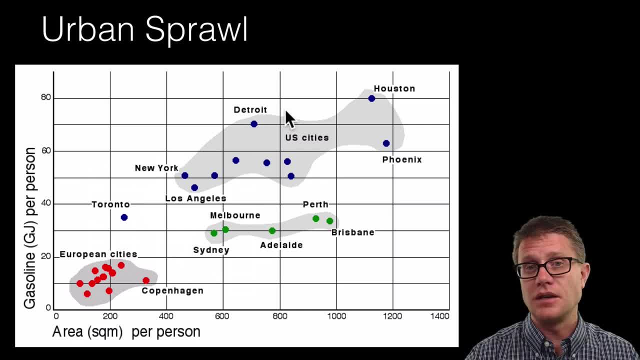 US we are going to be using more gasoline And so since cities in the US formed later than those in Europe, and also since we were using the automobile and we had increase in highway structure, we have had this sprawl be a larger problem in the US. It brings with 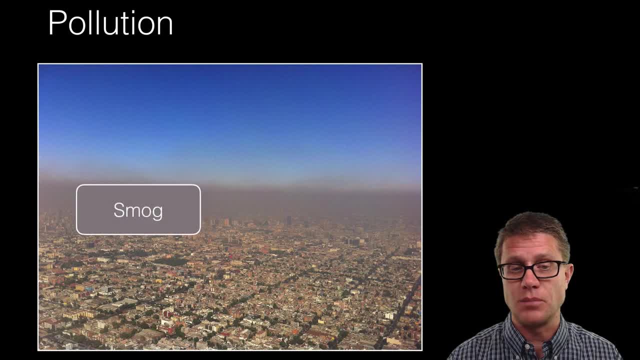 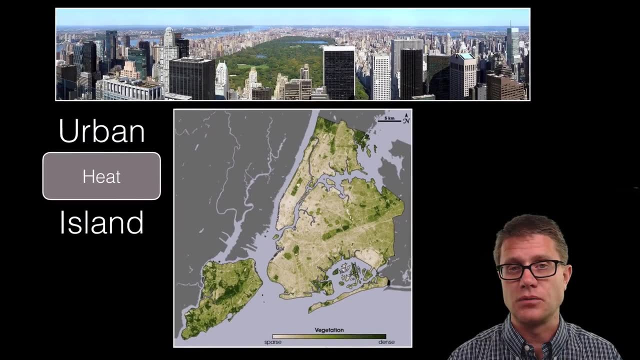 it problems in all cities. Pollution would be an example. So this is smog in Mexico City. We also get noise and light pollution and heat pollution. If we look specifically at heat pollution, we are seeing these heat islands where cities are, And so this is a picture. 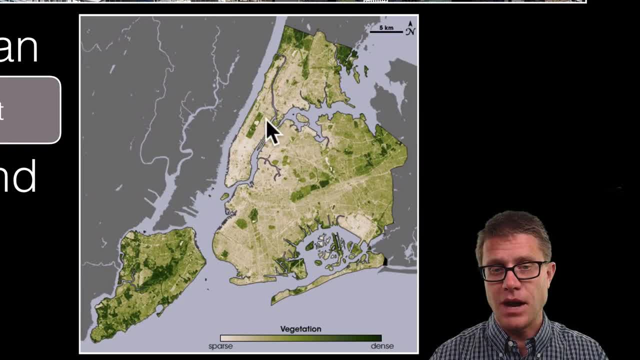 of Manhattan. This is Central Park right here, And then we are looking at a map down here, down on Manhattan. You can see Central Park right here And areas that are really green are areas that are rich in vegetation. But watch what happens if I now show you heat. 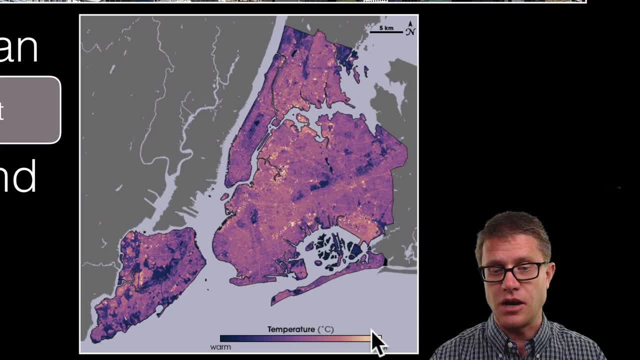 coming off of the land, You can see that we are going to have higher temperature, hotter temperatures, where we do not have that vegetation. So as we build up those cities, it is actually absorbing that heat and creating a heat island. And so how do we solve this problem? Well, 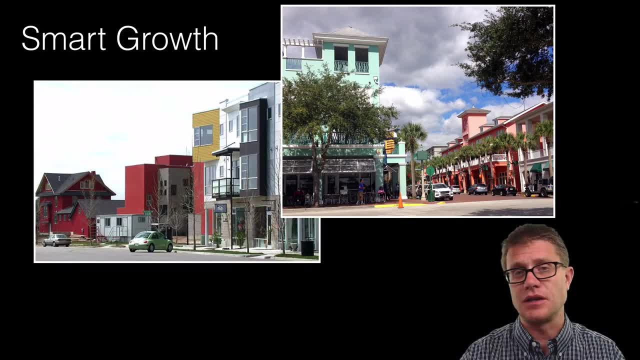 one thing would be to plant a lot of trees, But how do we return people to the city center? A lot of people are going around this idea of smart growth, And so we need to create desirable locations in the downtown: Walkable neighborhoods, Compact building designs, Sense. 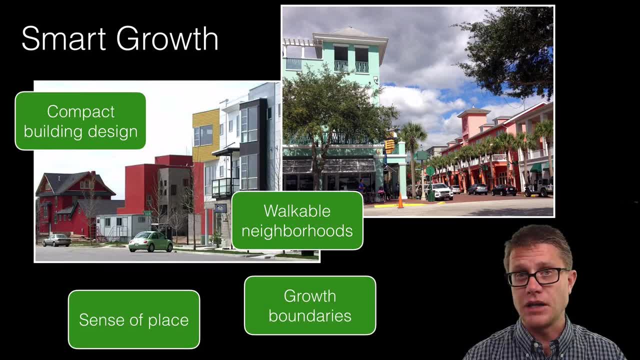 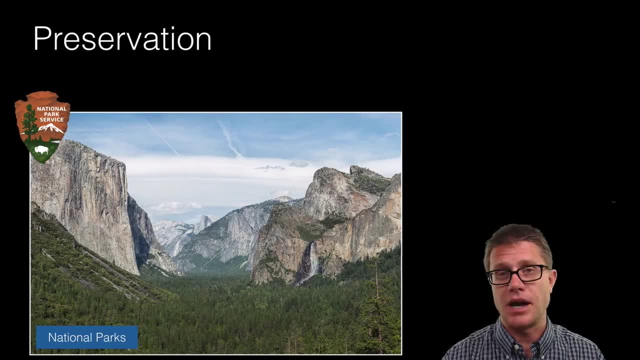 of place in the city, Growth boundaries, perhaps around the city, So we force people to stay within those settings. Now, there are pros and cons of all of these, But sprawl is definitely having some negative impacts Now outside the cities. we have also been trying to preserve 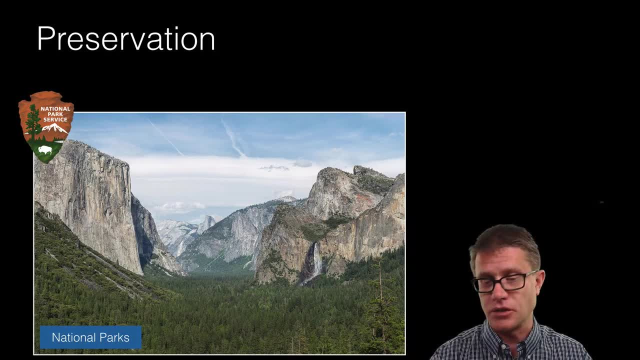 land. So the National Park Service was instituted And we have national parks like Yosemite and Yellowstone National Park. We have tried to protect the national parks. We have tried to protect the national parks. We have tried to protect the national parks. We have tried. 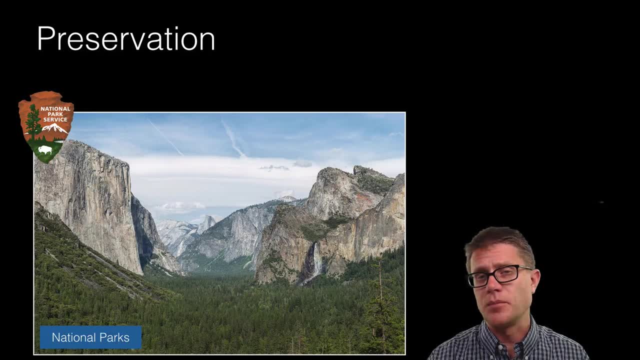 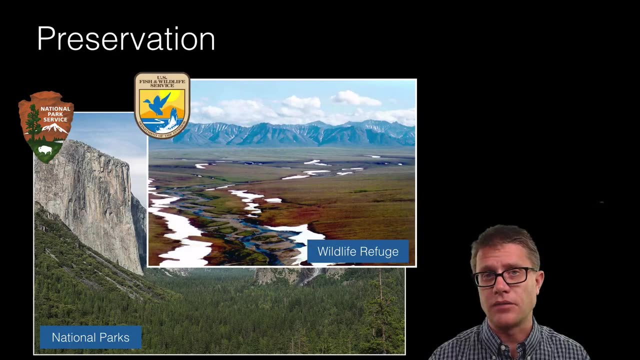 to protect this area for people into the future. I f you have ever been into a park, we still have roads there. We still have infrastructure run by the National Park Service. We also have wildlife refuges, So those are administered by the US Fish and Wildlife. So this is. 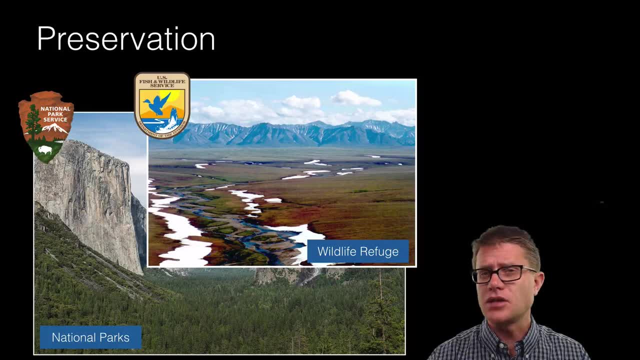 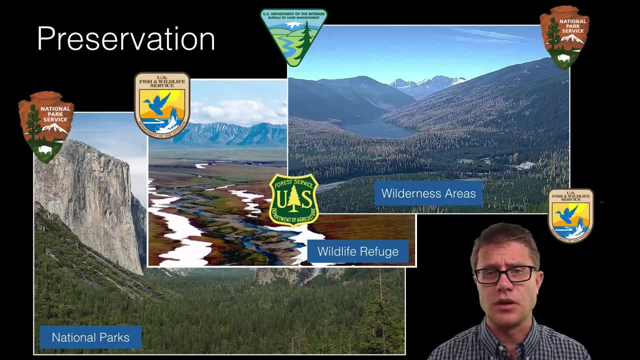 Anwar. This is in Alaska. its a National Wildlife Refuge. These are set up to protect specific species. In this case it is the Caribou, And then the strictest of constraints is the wilderness areas which are administered by all four of these entities. Inside a wilderness, 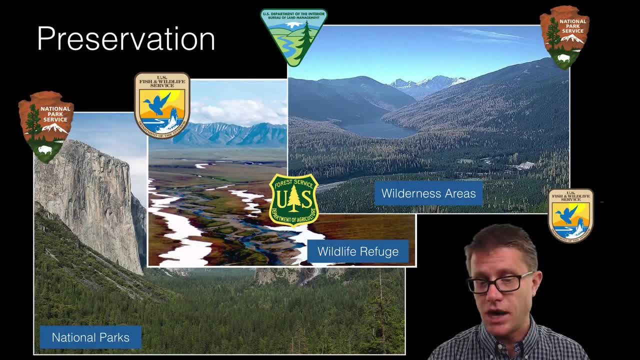 area. we try to connect them, those area that are already confined. You could use, or use any of those. In fact, we are going to ask the Green List of conferences if there are actually limit roads. the only way you can really get in is walking, riding a horse or by canoe. 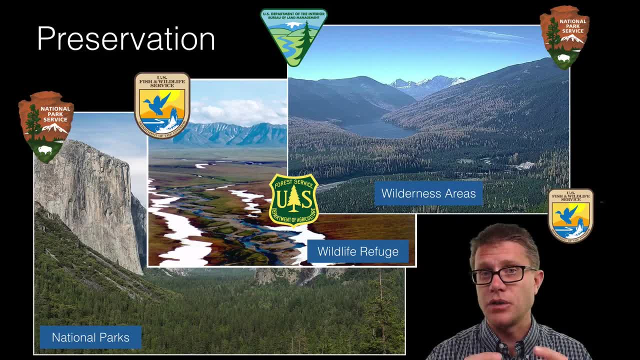 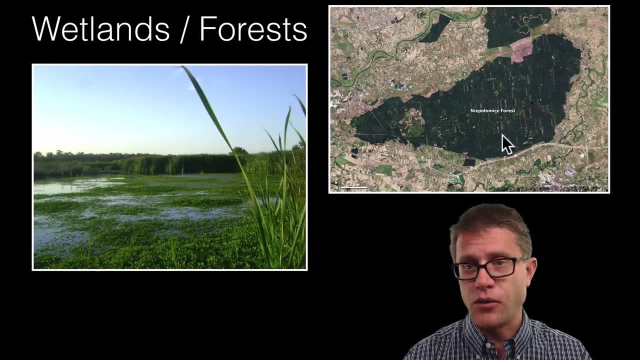 And so we do not have mining inside those wilderness areas, And so we are trying to protect these areas so they are not developed into the future, And we are also, on a micro scale, trying to protect wetlands around cities. This is a forest that has been protected in. 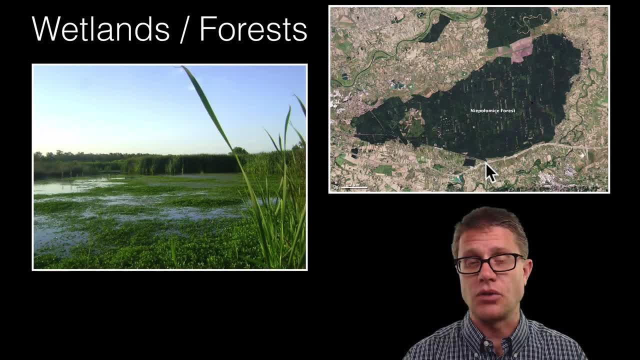 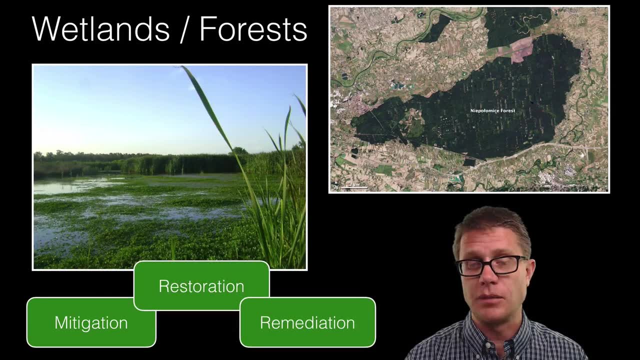 Poland since the 1300s. So if we put boundaries around that, we can, number one, mitigate it, so we do not have development into these valuable areas. We can restore them when they are damaged or remediate them. All of these are very big things that we can do around cities And 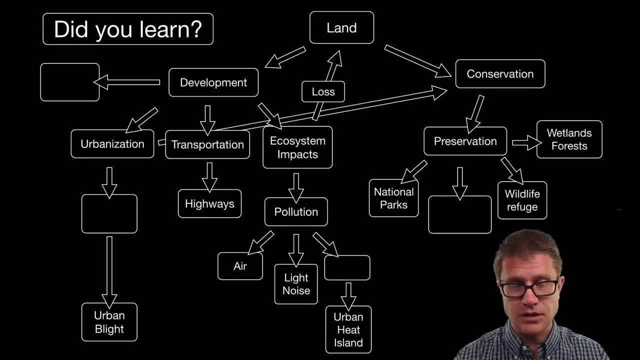 so did you learn the following? Could you pause the video to this point and fill in the blanks? Remember, development and urbanization can cause urban sprawl. That pollution could be air pollution, light pollution and heat pollution. We are trying to conserve our planet.